So what we've got is a lot of moist air being fed into a low-pressure system, which is quite intense. Now, very often, this cut-off low just wanders around and is unpredictable and causes heavy rain, maybe thunderstorms- I mean, the Landsberg Flood was one situation. 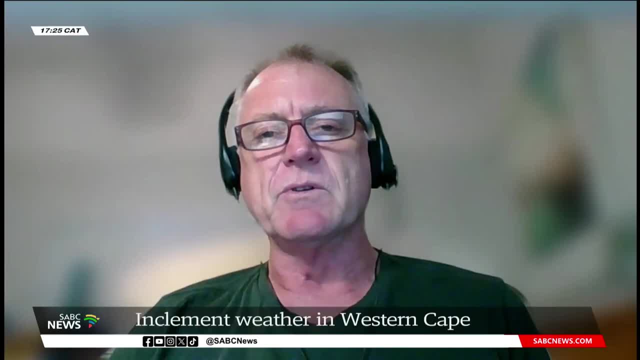 But what happened there? it was in a very much an enclosed catchment area and all the rain went down one river and washed away Landsberg. Generally speaking, the rain is steady, It can be very high, but it's not violent. What's happened now is this high-pressure cell, the isobars, which is the change of pressure over distance, have become very compressed and this leads to very, very high winds, And these high winds have fed into the cut-off low. So before the cut-off low even hit us, we had these very, very high winds, which didn't help with the fires that we had. We had those terrible fires before The rain actually arrived. Then the rain arrived, and now we've still got very high winds. and a cut-off low which is extending to the surface is very deep and very strong. This time we haven't had as much rainfall as other times. In the Heritage Day storm we had a lot of rainfall. This time we've only had 30, 40 millimeters, but we've had very, very high winds. 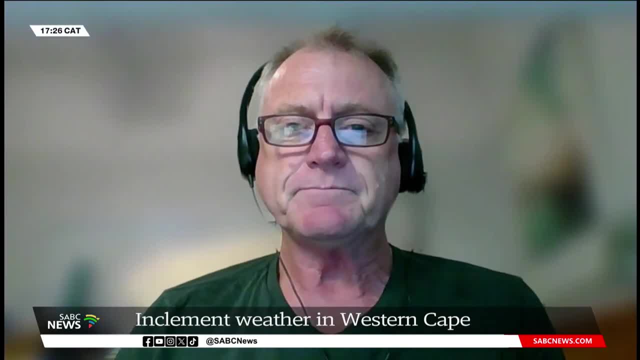 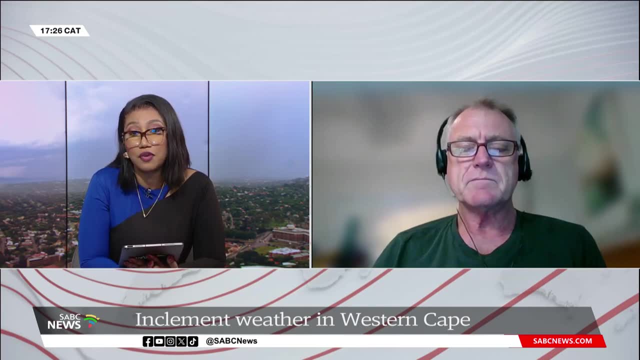 And those very high winds have caused the damage that you've seen. And what can we attribute to these almost extreme weather patterns? Because other experts have stated that, yes, conditions were actually fairly normal around autumn and perhaps the frequency would increase, as we're seeing, particularly in April. 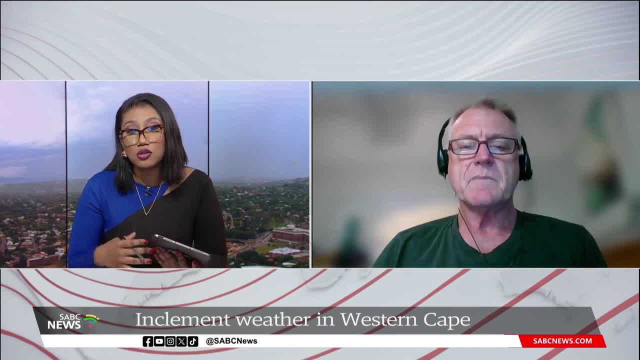 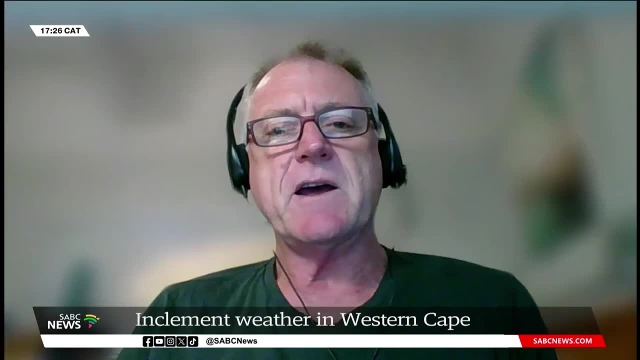 But many are still saying that the scenes are unusual. Are we not seeing more extreme weather conditions in the country of late, though? Yeah, that's a very debatable point. You've got to be very careful how you define an extreme condition. We've always had extreme weather. There have always been storms, There have always been floods, There have always been droughts. Cut-off lows are a regular feature, three or four times a year Sometimes. Sometimes they're in places that doesn't affect anybody and then we don't read about them. So when it does affect Cape Town- and this one was very squarely over the Western Cape- came into the countryside around about Friedendal in the West Coast and then moved across the Winelands and the Overburg and is now moving down the South Coast. 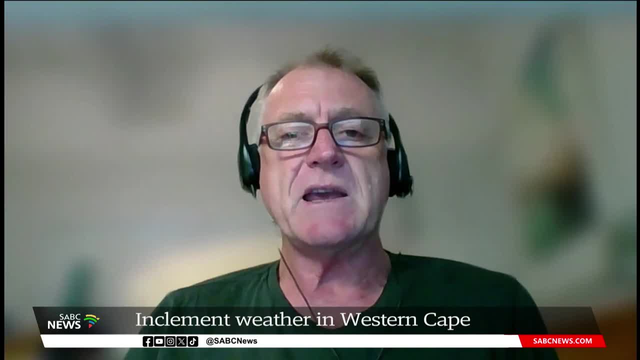 And, of course, it's a highly populated area. so we hear a lot about this and it becomes very, very newsworthy When these extreme events occur in places where people aren't living. we don't really hear about them. 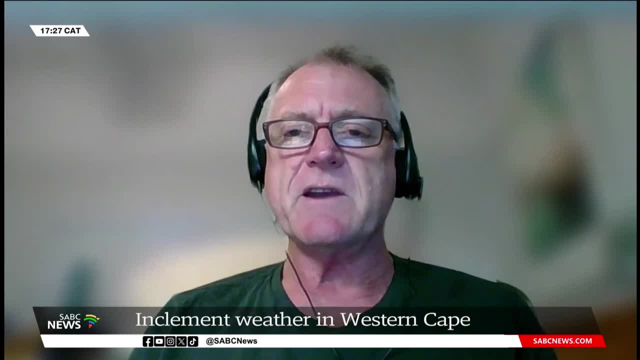 So it's quite tricky to say whether extreme events are increasing in frequency, but we do know that, due to climate change, the atmosphere is getting more active, It's more energetic, if you like, and we're seeing more cases of heavier-than-normal rainfall and possibly stronger winds. 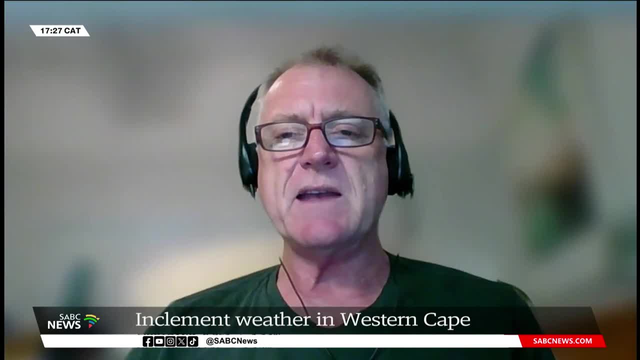 Now we cannot say that this event was due to climate change, but we can say that in the future our climate and our weather are becoming more variable. But that is not saying that we're all going to die and climate change is going to. you know, kill us in the next couple of years. We do not know what to expect this winter. We may get regular frontal rainfall in the Western Cape. We may get one or two cutoff lows. The cutoff lows are likely to have heavier rainfall. and possibly stronger winds than the regular frontal systems, But we know the frontal systems can be very violent. We can get very, very strong northwesterly winds blowing over the peninsula, damage in low-lying areas, flooding also in areas where people are too close to rivers. or where there are areas that are low-lying And that weather can extend right into the country. So it's completely normal for this time of year for us to have the change from summer to winter. As we said before, this is what's happening in the country. 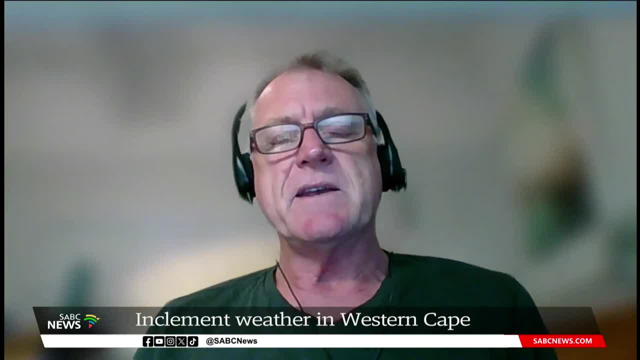 The summer rainfall region, rainfall is becoming less and less, and the winter region rainfall is becoming more and more. We just hope that we don't have excess rain, whether it's in floods or whether we have too little rain in terms of droughts. What we'd like is a sort of regular normal rainfall, but that very seldom happens. We have as many droughts here, We have wet years and we really don't know what's going to happen. but we have to be prepared. 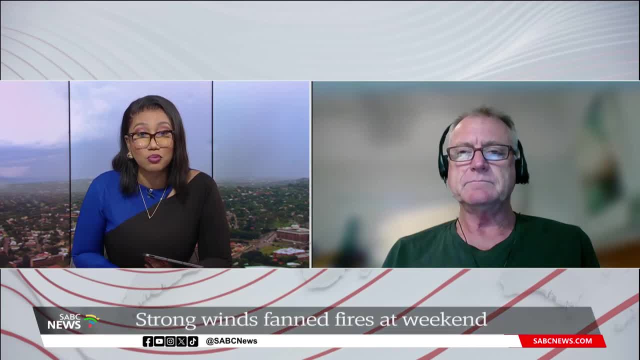 Now it's quite comforting, Doctor, that experts say we shouldn't panic, because with just those visuals many of us were panicking and probably looking to attribute this to climate change. But, as you say, that's not necessarily in this particular instance. 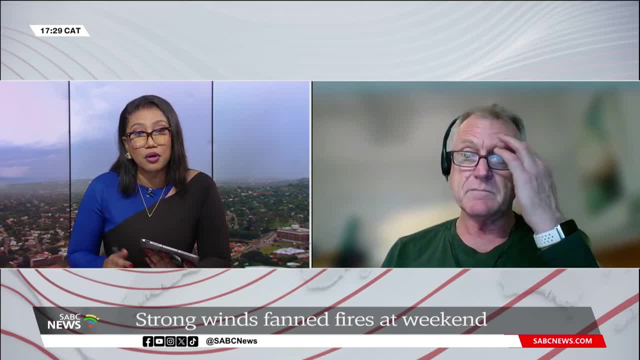 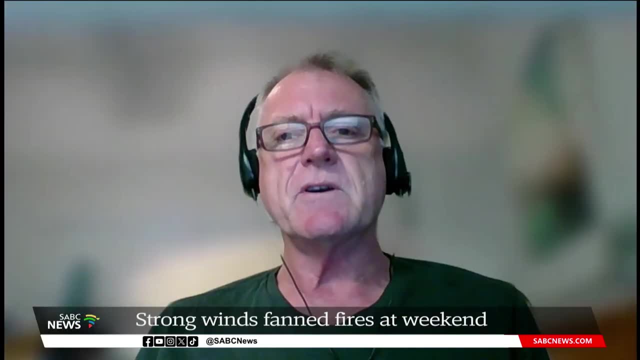 But can you talk us through the impact of such weather on agriculture? Yeah, so remember that there's various different types of agriculture. Right now we're going into the winter rainfall region, So the Western Cape, they're going to be planting weeds. 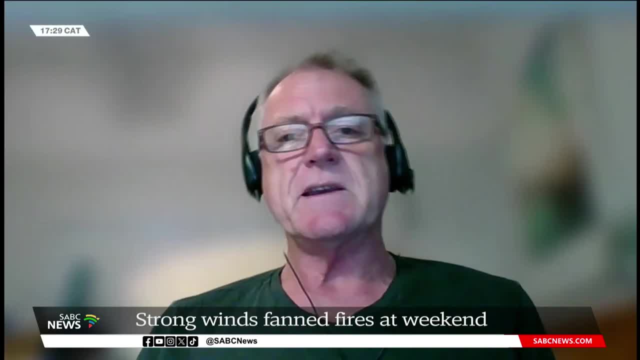 wheat. this month and next month The fruit farmers are still harvesting. The apple farmers must have had a torrid time, because there's some breeds of apples or types of apples that are still on the trees and haven't been picked yet, And I'm wondering if any are still left on the trees. So that's an important thing, that if you're about to harvest in a wind like this and the rain doesn't really bother it too much, but the wind like this can cause severe damage. We've seen images of tunnels where they grow, berries being blown away. Those sort of high value crops are very susceptible to high winds and high rains, like we've been having. The wheat farmers, on the other hand, are quite happy There's been some rain. it wets the soil and they're getting ready to plant. 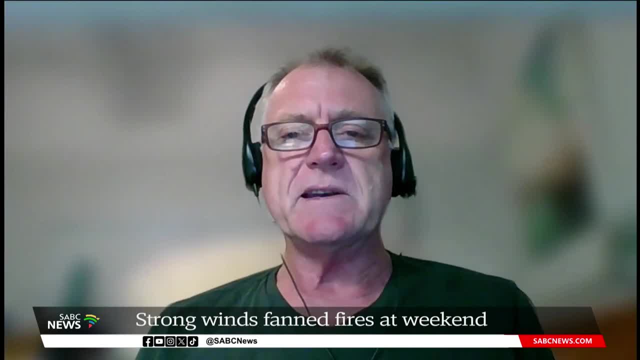 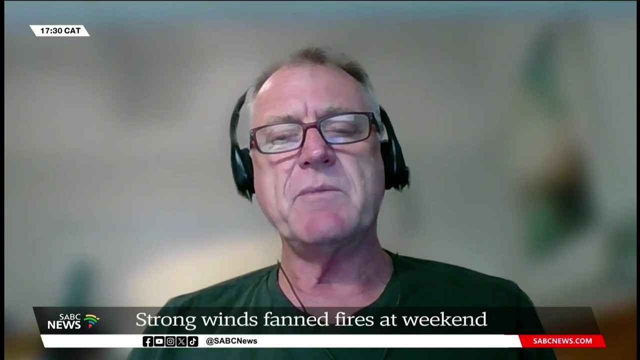 The wind doesn't affect them at all- Well, when I say at all. obviously it can blow some of their soil away, But most of them are practicing conservation agriculture and that's protecting the soil. When we go inland, we're seeing that maize, particularly, is about to be harvested. 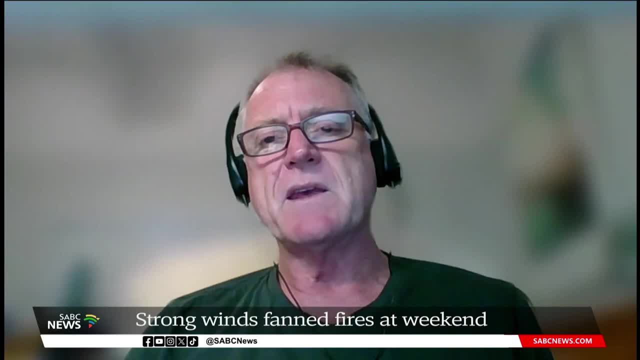 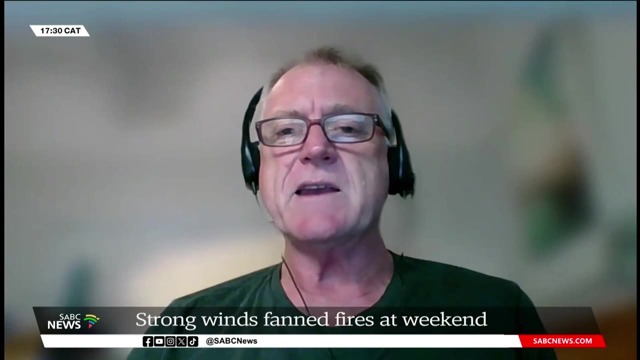 Well, it's drying at the moment and it's coming into harvest. The wind can cause some lodging. The wind can cause some troubles there. A late rain in early winter can also cause some fungal diseases. So anything that's out of the normal where we're growing crops that are designed for a specific climate- can cause some damage. The agricultural infrastructure normally can withstand the kind of winds- the barns, the silos, things like that- And machinery is usually kept out of the storms and out of the wind, So that should be OK. But it is damage to crops, especially high value crops, that are being harvested right now. 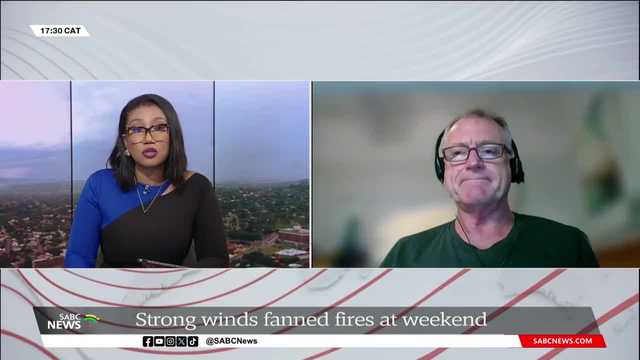 Doctor, thank you very much for your insights this afternoon. That was Dr Peter Josten, climate scientist at the University of Cape Town. 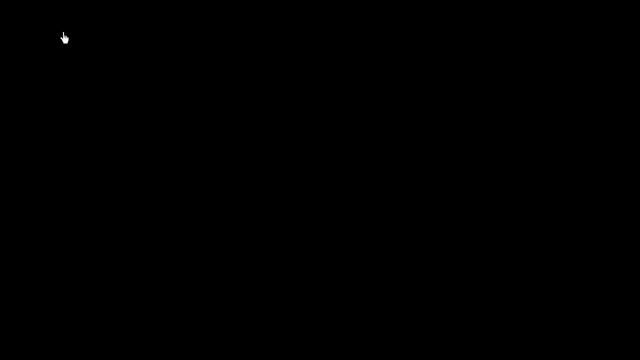 Whenever we talk about money, the amount of money is not the only thing that matters. What also matters is when you have to get or when you have to give the money. So to think about this or to make it a little bit more concrete, 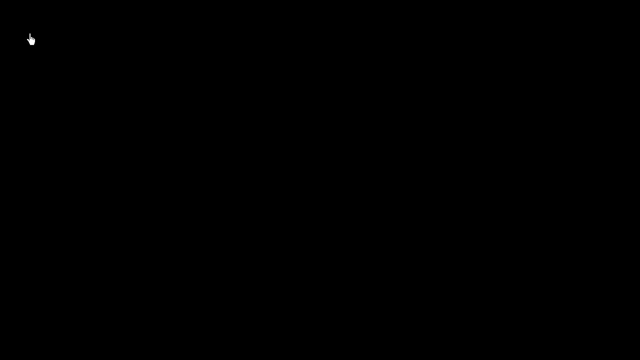 let's assume that we live in a world that if you put money in a bank, you are guaranteed 10% interest, 10% risk-free interest in a bank, And this is high by historical standards. but it'll make our math easy.